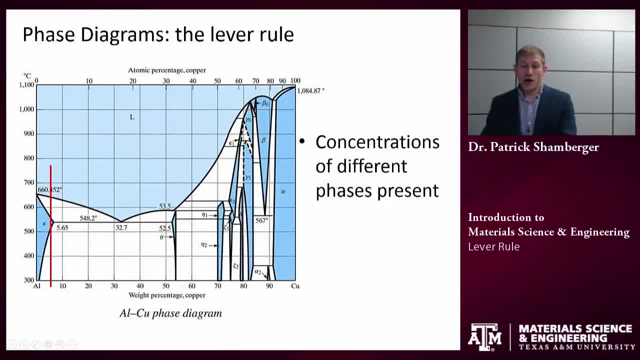 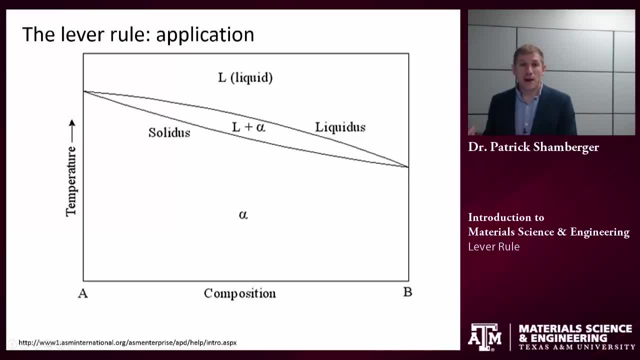 in this case, is perfectly applicable to a more complicated system. We're going to, having said that, we're going to- start off with a little bit easier system. So, again, this is a binary isomorphous Bayes diagram. Now we use the lever rule when we want to know what. 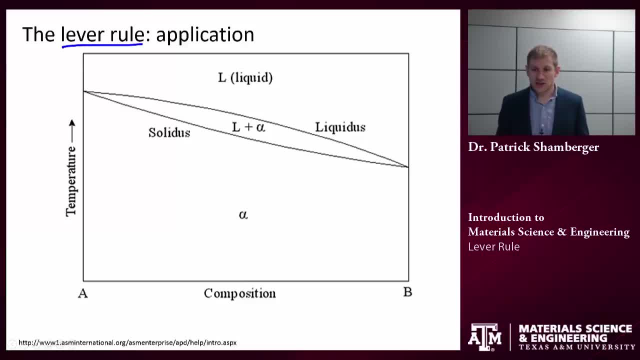 is the concentration of the different phases present. So how much, in this case, how much solid alpha and how much liquid is there? And the phase rule, the lever rule, allows us to calculate that. So let's do an example. Let's say the 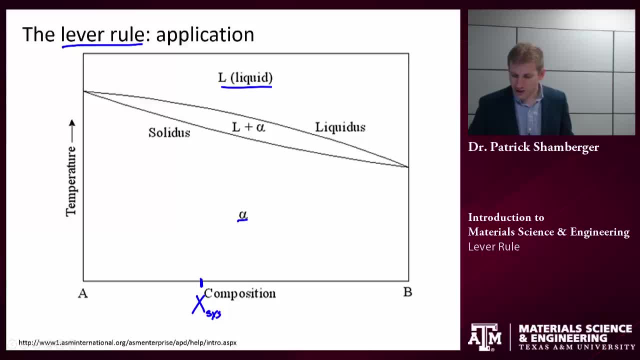 bulk composition or the system composition is. well, it looks like 40% B, component B. As a side note, sometimes this is called bulk, sometimes it's called the system, sometimes it's called total or the whole. In all these cases, we're picturing a system being a box. 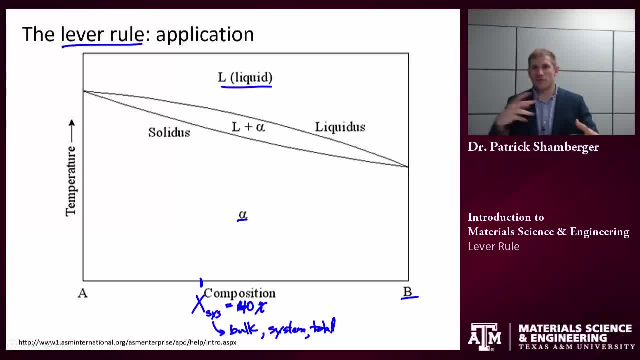 that we have some material in. We want to know what is the composition of everything in that box. Okay, At some temperature up here we are in the two phase region, And so the first thing that you want to do when you're in the two phase region is draw a tie. 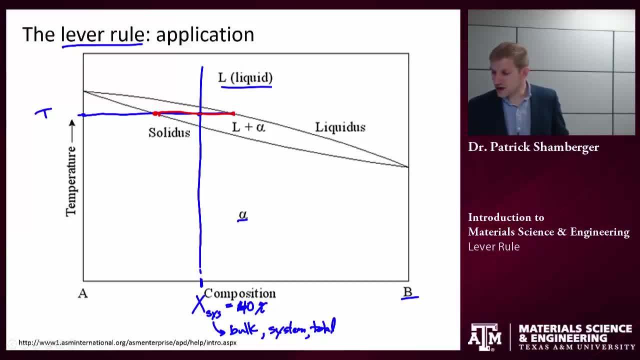 line, And this tie line is going to give us important information. It tells us what is the composition of the solid present and what is the composition of the liquid present. Okay, In order to to apply the phase rule, we need all of these numbers. So this liquid. looks like they are more than our total. So let's draw a solid number, for instance, and let's change this number up. So let's Blog1 column over So that we can figure out what the number is off than the number of followers is. We've got a two component formula by the. 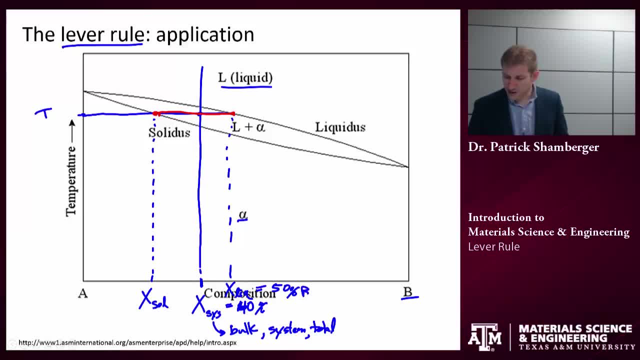 it looks like it's about 50% component B, The solid. maybe, just to do the math easier, we'll say it's about 30% component B. Okay, so to apply the phase rule, I need to know three things. 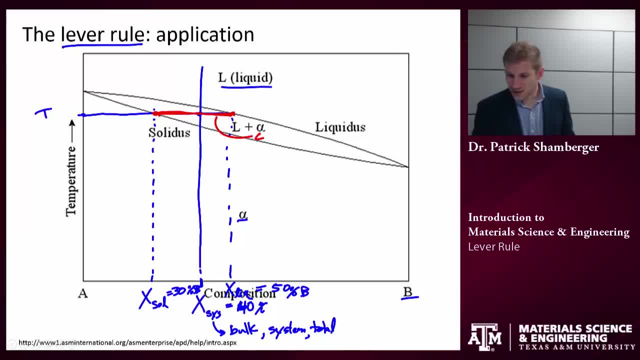 I need to know this overall length. I'll call that C. I need to know this length, I'll call that A. And I need to know this length, and I need to know this length and I'll call that B. So in this case, A is given by the difference. 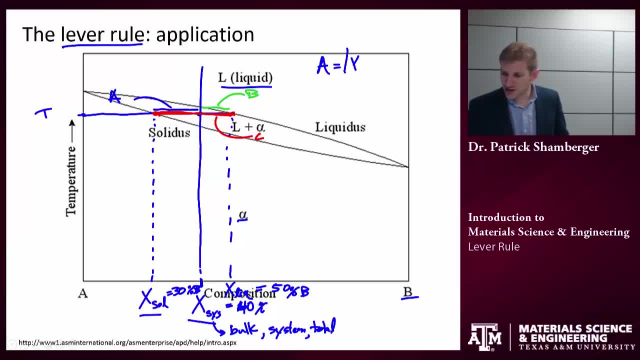 between the system and the solid composition, And so we usually look at the absolute values. that way, we don't have to worry about signs in this case. So the system composition I said was 40%. Let's start to use fractions or decimal fractions. 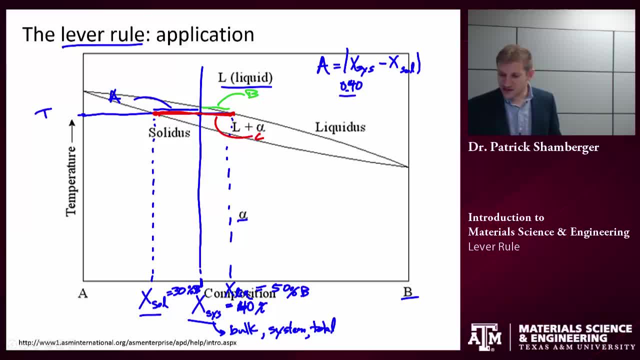 because that's a little bit easier. The system is .4, the solid composition is .3.. So A equals 0.1.. Okay, what about B? In this case, B is .5 minus .4.. That is 0.1.. 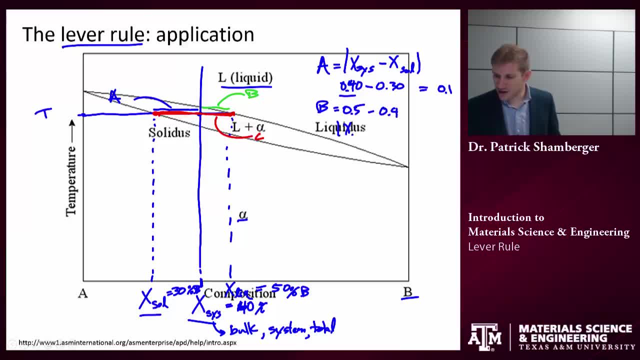 That is 0.1.. That is 0.1.. It's the liquid composition minus the system. So B is the length from here to here, And that also equals .1.. Finally, C is this overall difference. So C is the composition of the liquid. 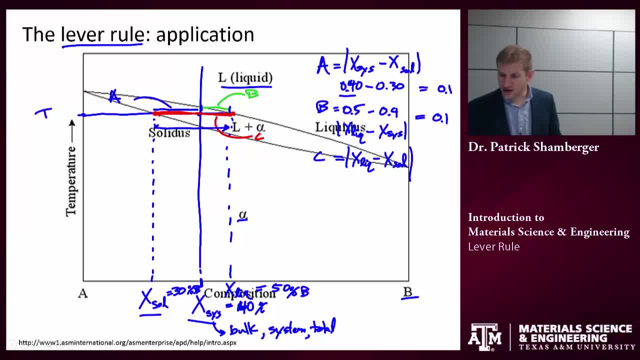 minus the composition of the solid, And so in our example that's 0.5 minus 0.3 equals 0.2.. So if I'm applying the lever rule, I'm asking how much is there of some particular phase? 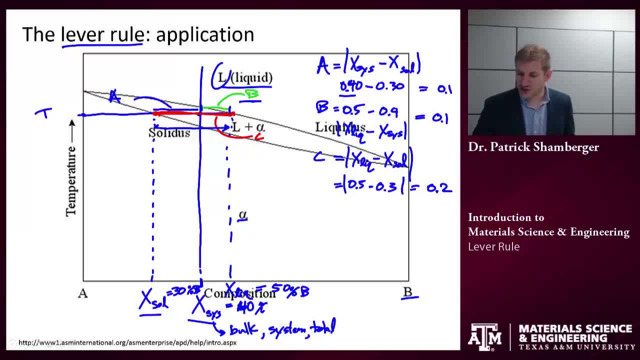 So let's ask the question about the liquid first. So how much liquid? In this case, I would take the fraction A over C, And so, using the numbers I've calculated here, that's 0.1.. And so, using the numbers I've calculated here, that's 0.1.. 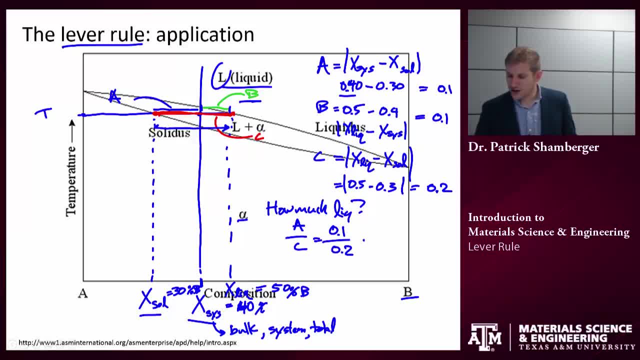 And so, using the numbers I've calculated here, that's 0.1.. And so, using the numbers I've calculated here, that's 0.2.. And so, using the numbers I've calculated here, that's 0.1.. 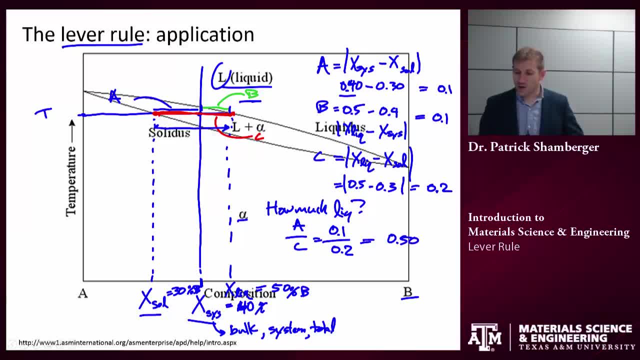 And so there is 0.5, or 50. weight percent. mass percent mass fraction. sorry of the system is liquid. mass percent mass fraction: sorry of the system is liquid. How about the solid? How much solid is present? 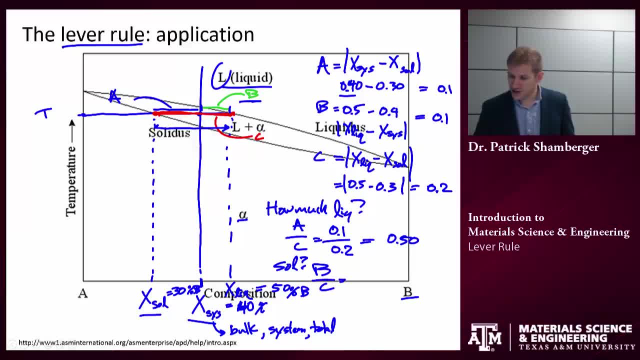 That's given by B over C. Again that equals 0.1 over 0.2, 0.5.. Again that equals 0.1 over 0.2, 0.5.. Again that equals 0.1 over 0.2, 0.5.. 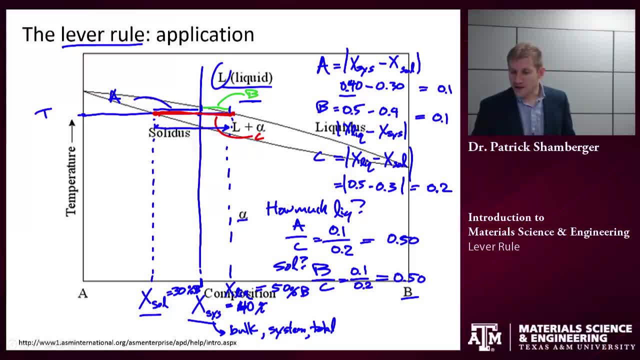 So what I've said is, for these numbers, there is .5 mass fraction of liquid and .5 mass fraction of solid phase alpha present. That's about right, because this line is about in the middle of my composition. In reality, this number probably was a little bit higher than it should have been. 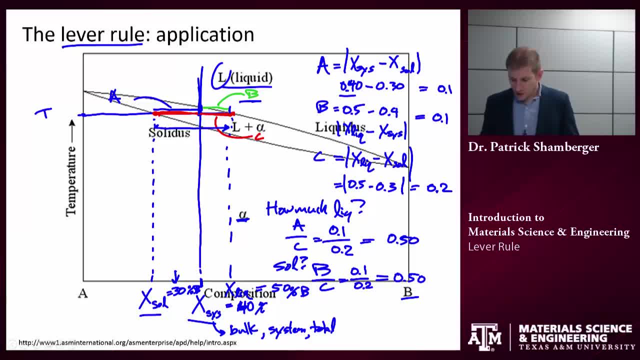 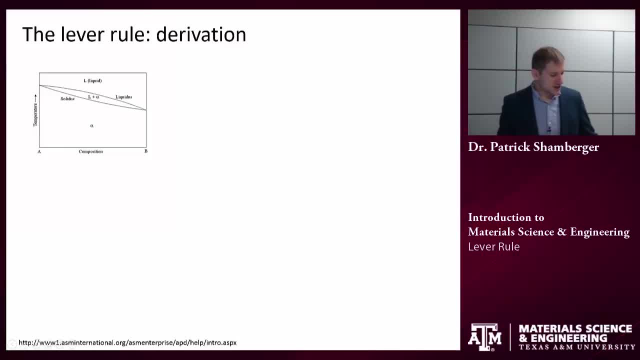 But this is how we apply the lever rule. Okay, let's talk about derivation. Where does the lever rule come from? I told you before it's related to mass balance. So let's look at a system And again at some composition of the system and some temperature. 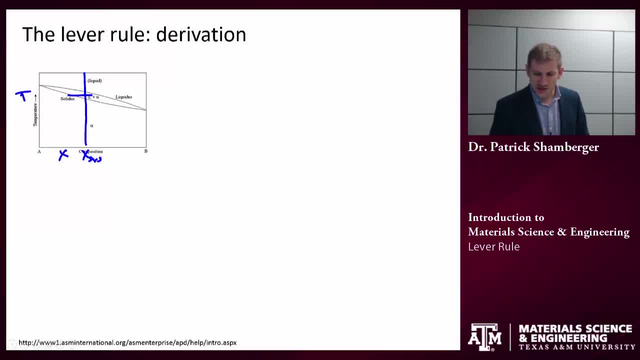 And again, let's use these terms that I defined before- What is the composition of the solid, the composition of the system and the composition of the liquid? So I will say x solid, And this is in terms of B. I could do it in terms of component A as well and get the same exact answer. 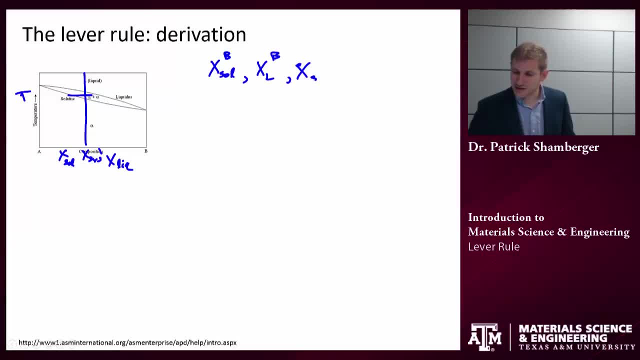 x liquid and x system. Okay, let me also define a couple other variables, And I'm going to use w for a mass fraction. What is the mass fraction of phase alpha And what is the mass fraction of the liquid present? And I know that the mass fraction of these two added together equals 1.. 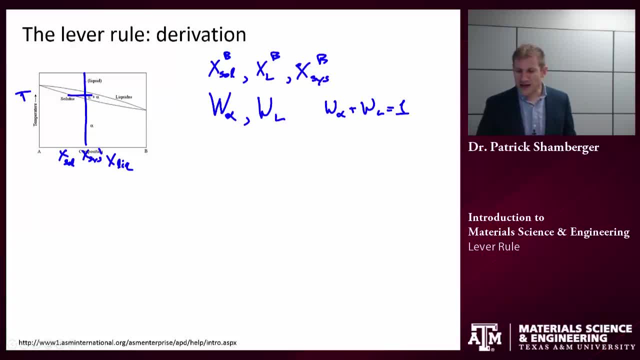 Okay, so what does the mass conservation tell us? Well, the composition of the solid. just to be consistent, we're going to use alpha here. The composition of alpha times the mass fraction of alpha, plus the composition of the liquid times the mass fraction of the liquid. 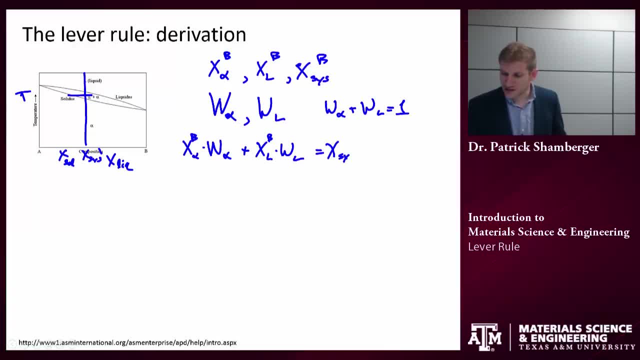 is going to equal the composition of the system times the mass fraction of the system, which is just 1.. So this is basically a mass balance equation. Okay, I can substitute this relationship in for either of these two variables. Let's say I replace w sub alpha. 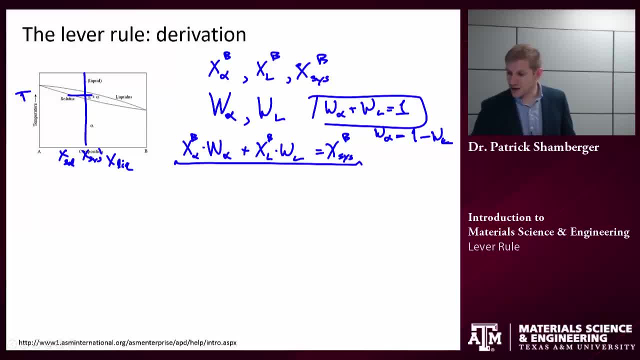 with 1 minus w sub l. So the mass fraction of solid present equals 1 minus the mass fraction of liquid present. So I'm going to substitute that back in here: x, alpha B. Okay, so I'm going to get something like this: 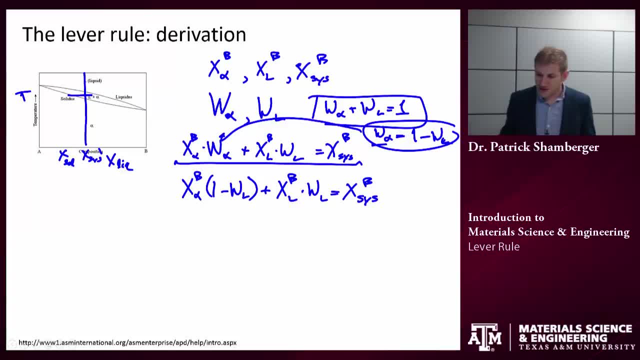 Now the next steps are basically simple algebra, but I want to solve for w sub l. The whole purpose of this is to calculate the mass fraction of liquid, or phase alpha, from the compositions of those different phases, And I encourage you to work through this yourself. 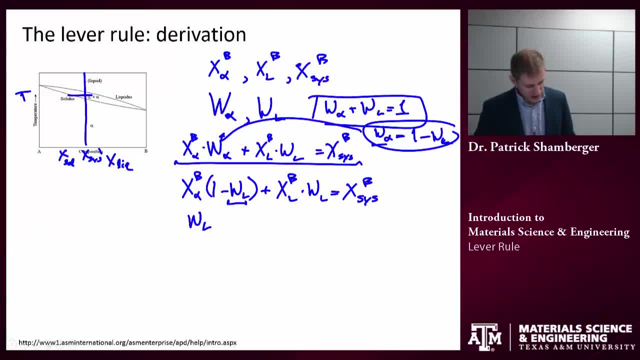 but what you'll find is the mass fraction of liquid equals composition of the system. put absolute values on here, minus composition of alpha, over composition of liquid, minus composition of alpha, And again this is all relative to component beta. I could repeat this calculation for component alpha. 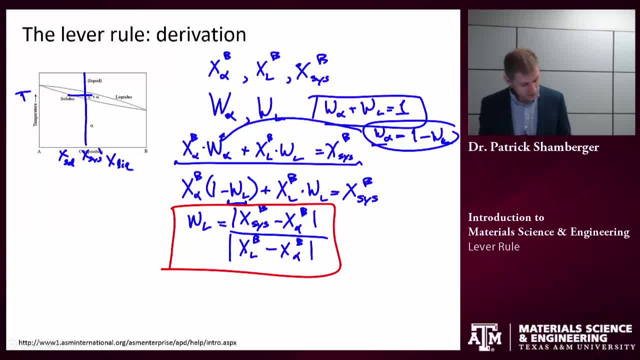 and get exactly the same result. And this is this ratio that we used in the previous figure. So system minus alpha- Again, this is alpha here. So system minus alpha is this distance. I believe we called that, Yeah, So we called this A. 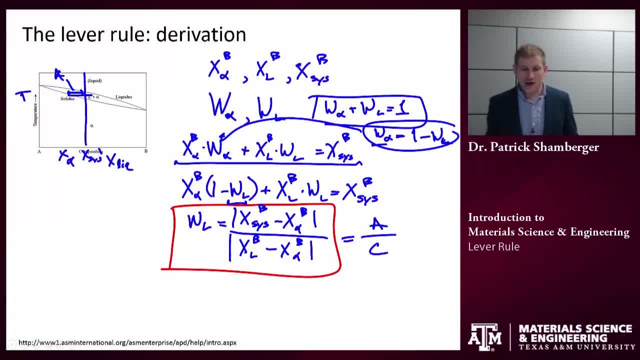 Liquid minus alpha is the whole length. So A over C. Okay, so this is where the lever rule comes from mathematically. Some people like to see that derivation. The final thing we're going to do is just a quick little sanity check. 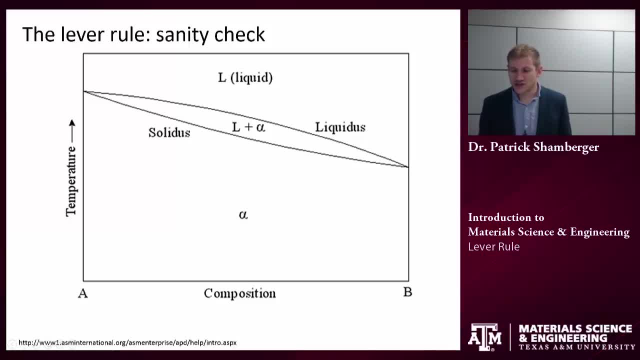 And I encourage you always to do this when you're asking questions about concentration- of different phases present, And so I'm going to Just to make sure I'm getting the point. I wanted to start up here. Let's say, my system composition is this: 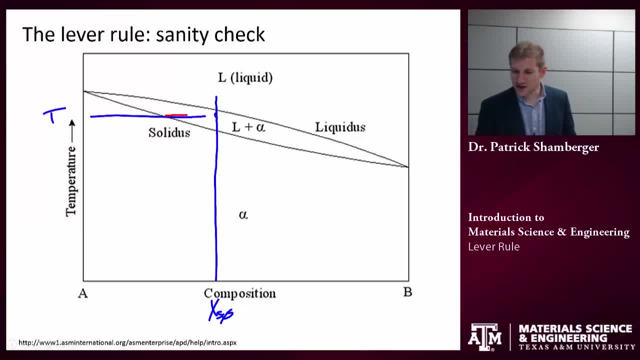 and my temperature is this. Again, the first thing that I always do if I'm in the two-phase region is I draw my tide line. Okay, now you can notice. here's my composition of liquid, Here's my composition of alpha. Now the composition of the overall system. 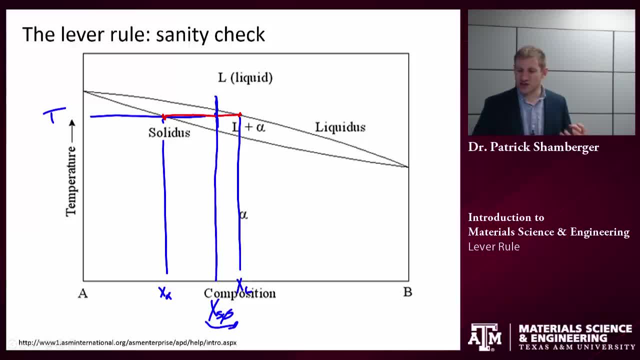 in this case, is a lot closer to the composition of that liquid phase. So for the only way for this to make sense, there needs to be more liquid than there is solid. Think about that for a second. If the composition of the system is closer to the liquid case, 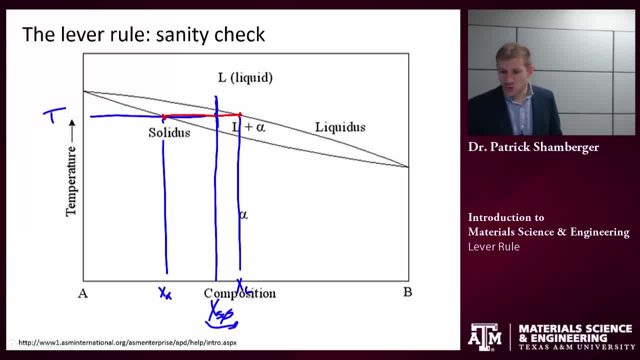 there needs to be more of that liquid present. So when we look at our different, our different lengths involved in the lever band, I drew this intentionally so that A is significantly longer than B And remember the fractions are either A over C or B over C. 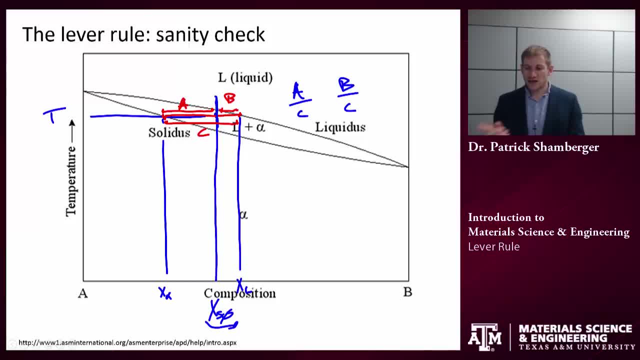 And the most common mistake that students make is mixing up which one of those refers to how much liquid is present and which one refers to how much solid is present. But remember what I just said. I know that there's more liquid present in this case. 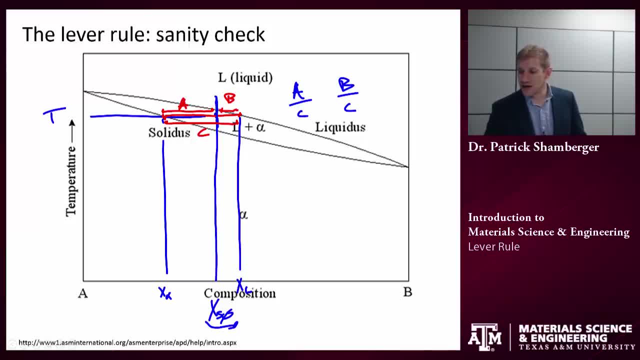 And so A over C. you can tell just by looking A over C is going to be larger than B over C, And so A over C refers to the liquid. So I would call this a sanity check. Look at the system, See if the ratios that you're calculating make sense. 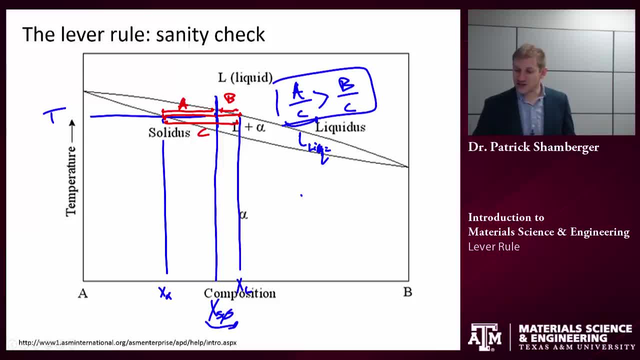 These should always be. if I'm calculating fractions, it should always be between 0 and 1.. And whichever phase I expect there to be more of in this case, I expect there to be more liquid. that's going to give us that one is tied to A over C.